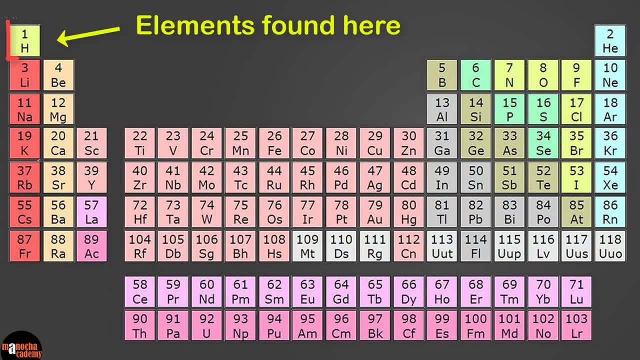 So you'll find elements such as hydrogen carbon nitrogen on the periodic table. So you'll find elements such as hydrogen carbon nitrogen on the periodic table. You won't find compounds such as water or carbon dioxide. Now, elements are the simplest substances in chemistry. 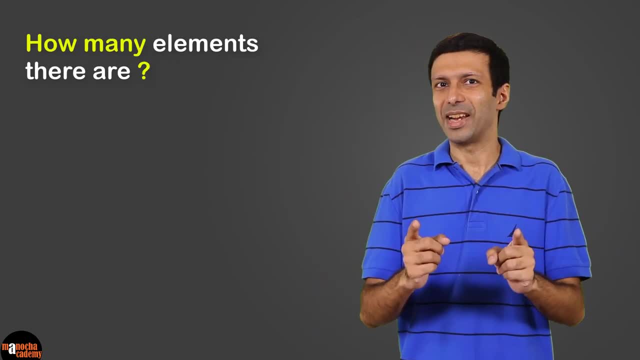 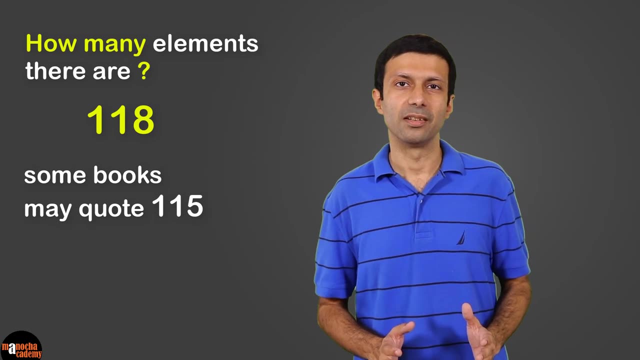 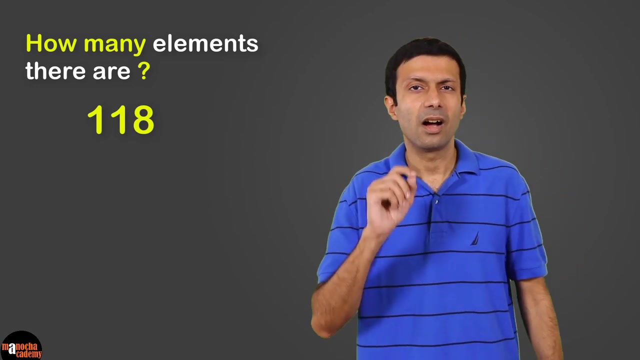 Do you know how many elements there are? That's right, 118 elements. Now, some books may quote a lower number, such as 115, because probably a few elements are still under research, But if you check up Wikipedia, it says that 118 elements have been found. 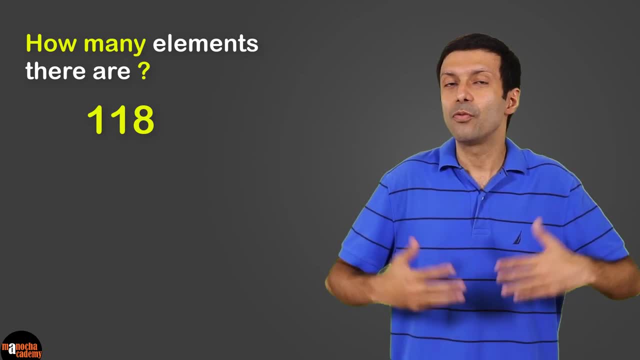 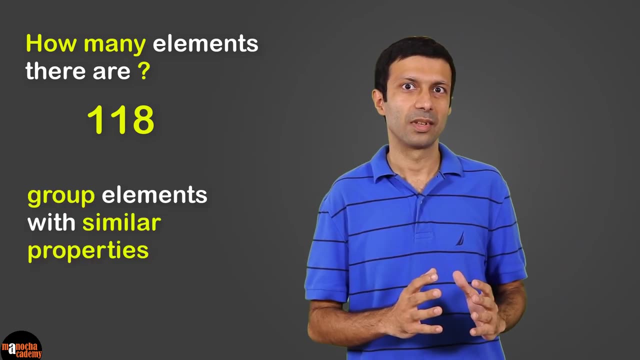 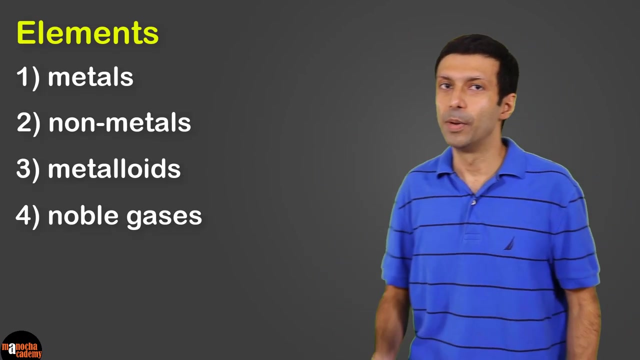 But if you check, up Wikipedia, it says that 118 elements have been found. So that's a lot of elements to study, right? So it makes sense to group elements having similar properties together. For example, we can divide the elements as metals, non-metals, metalloids and noble gases. 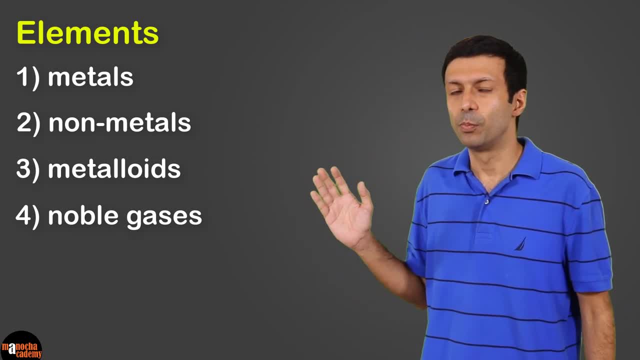 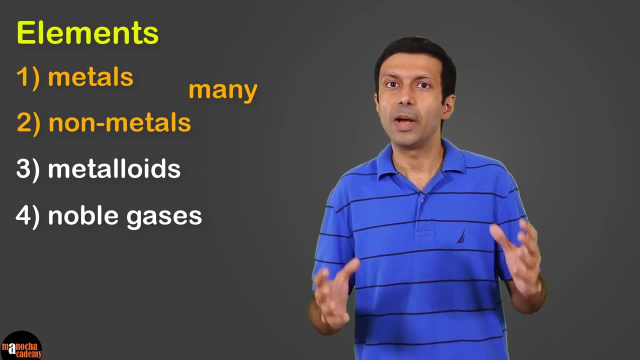 But the problem with this approach is that these categories are too broad. There are too many metals and non-metals, So many scientists were working to group elements having similar properties, But keep in mind not all the elements had been discovered. 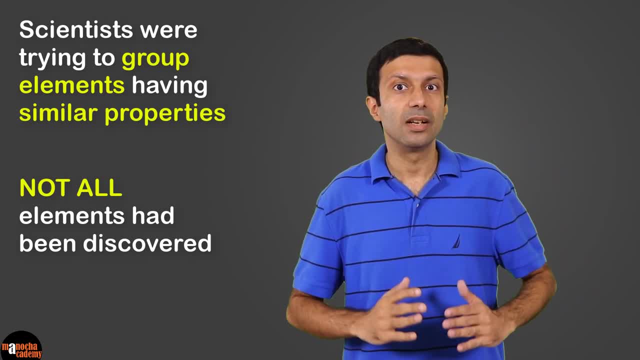 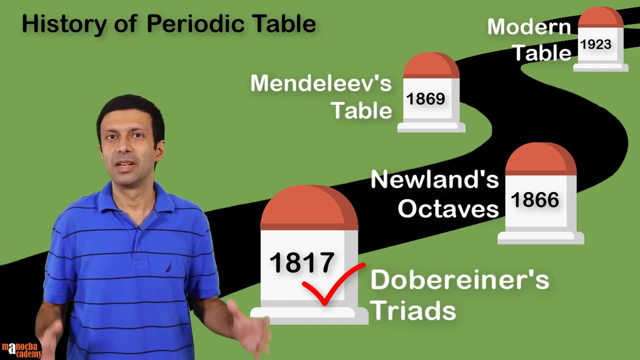 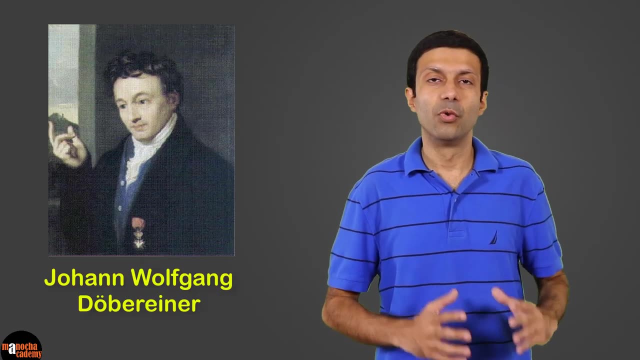 They were working with only the elements that had been discovered at that time. Let's go back in history to 1817 and look at one of the initial attempts to classify elements. These are famously known as Doberinier's triads. Johann Wolfgang Doberinier, a German scientist, was the one who discovered them. 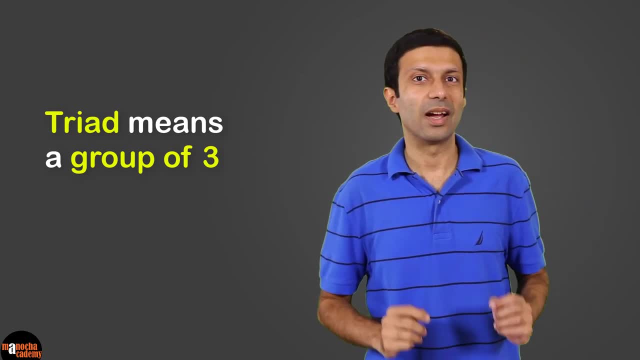 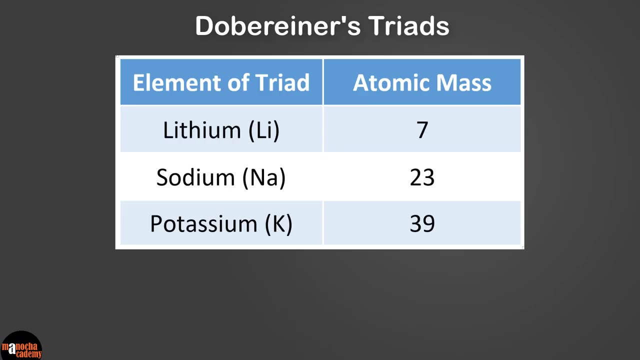 Triads are the elements that are the most important elements in chemistry. Triad means a group of three, So let's take a look at the triads made by Doberinia. Here is one of the triads made by Doberinia. 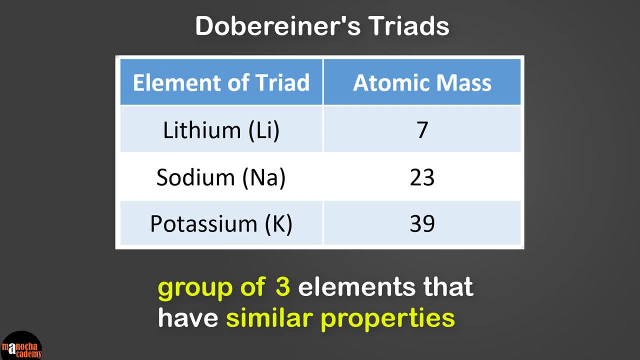 It's a group of three elements that have similar properties, For example, the elements lithium, sodium and potassium. here are metals. They react with water to form alkalis and hydrogen gas. These three elements have valency 1.. One special thing about the Doberinia triads is that if you write the elements in order, 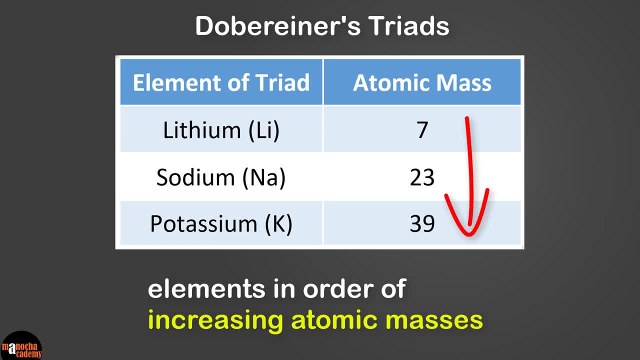 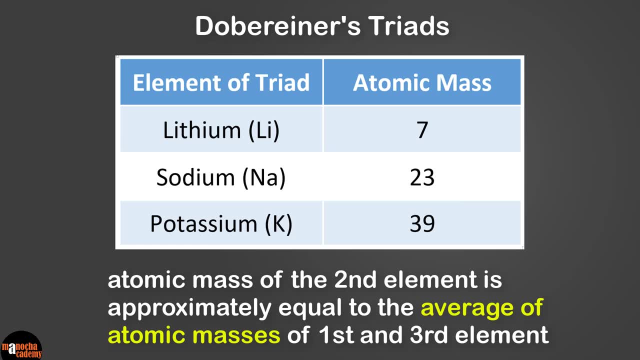 of increasing atomic masses like this. then the atomic mass of the second element is approximately equal to the average of the atomic masses of the first and third element. Let's take the average of the atomic mass of the first element, lithium, and third element, potassium. 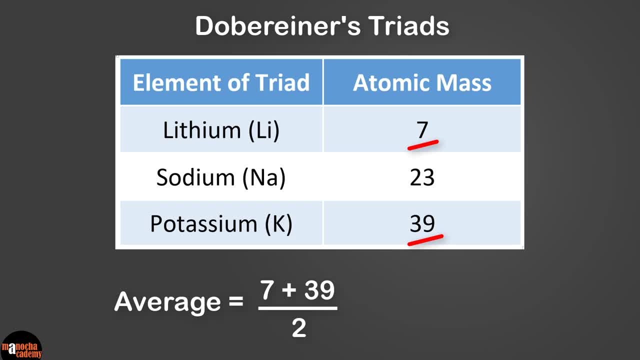 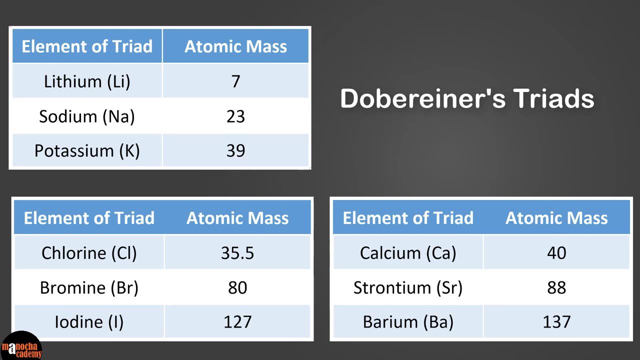 So we'll get 7 plus 39 by 2, which is 46 by 2, and that's equal to 23.. And this is the atomic mass of the middle element sodium. Here are two more triads that Doberinia discovered. 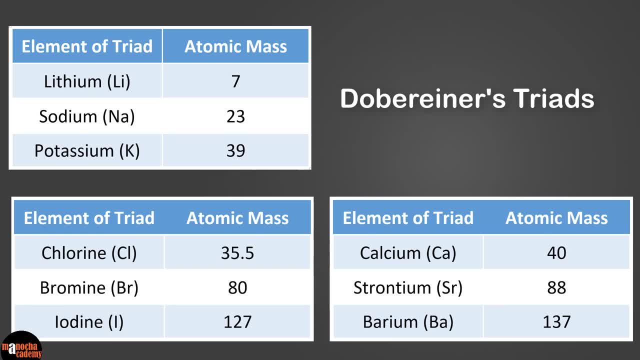 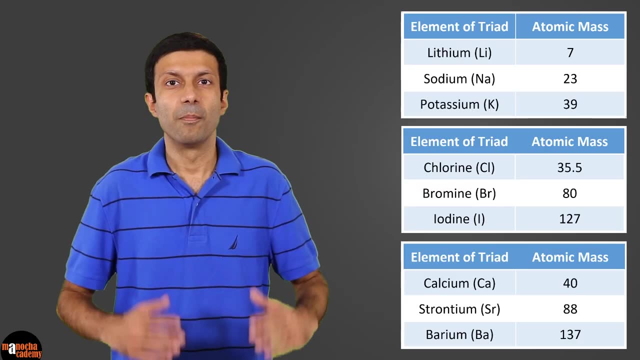 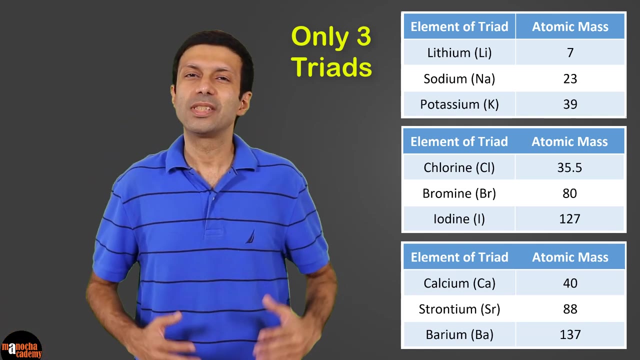 The elements in the triads have similar chemical properties. Again, if you take the average of the atomic masses of the first and third element, It is approximately equal to the atomic mass of the second element in the triad. But Doberinia could identify only these three triads from the elements known at that time. 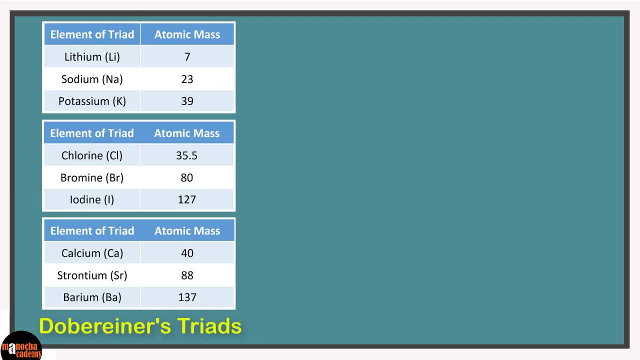 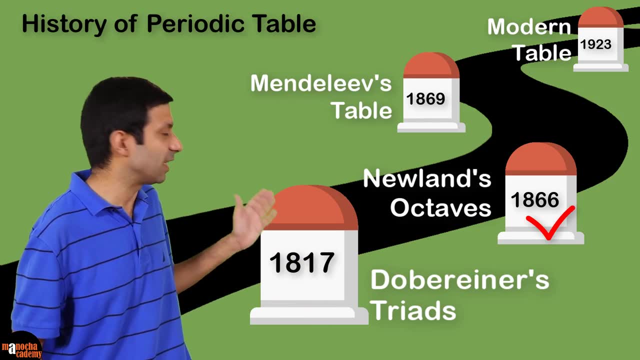 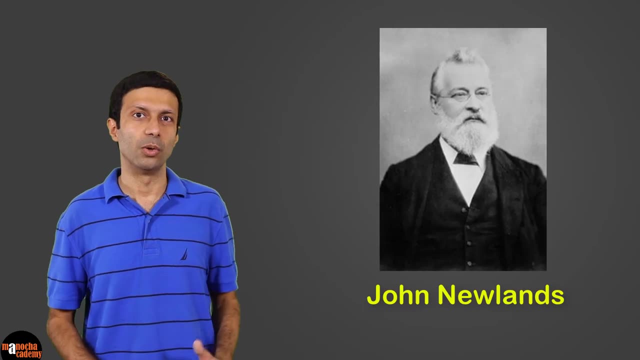 So his classification wasn't so successful. Let's place Doberinia's triads on our concept board. Now. let's move ahead to 1866, to Newland's law of octaves. This was proposed by an English scientist, John Newlands. 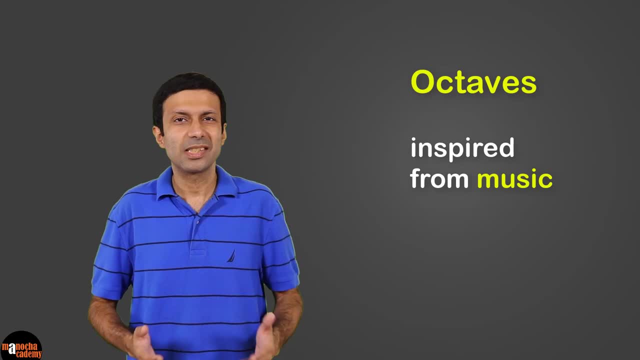 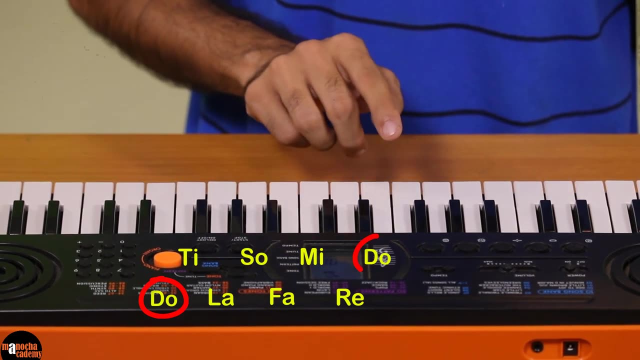 The word octaves is inspired from music, So, just like we saw on the keyboard, Do Re Mi Fa Sol La Ti Do. The eighth note is a repetition of the first note. Similarly, Newlands observed that when he arranged the elements in their order of the 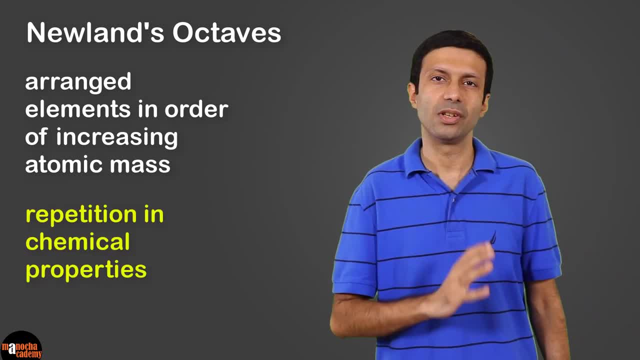 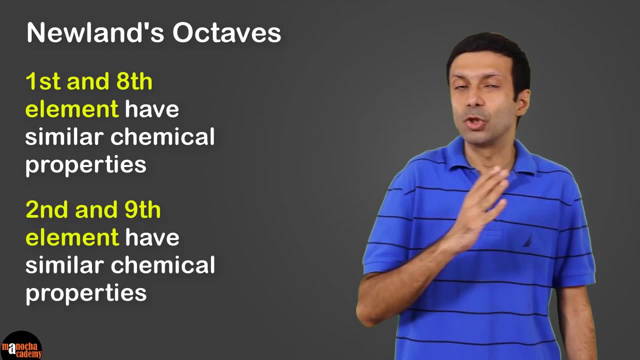 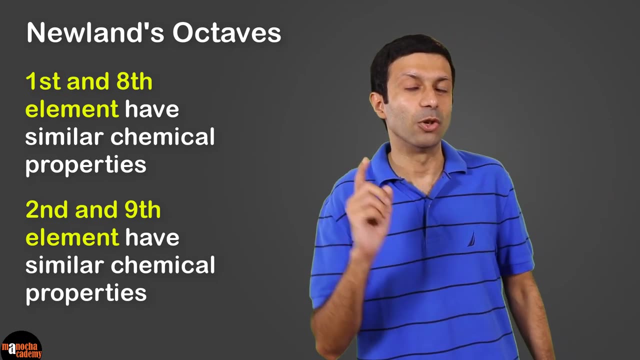 increasing atomic mass. he saw a repetition in chemical properties, where the first and the eighth element have similar chemical properties, And so do the second and the ninth one, And so on. So let's take a look at the table made by Newlands. 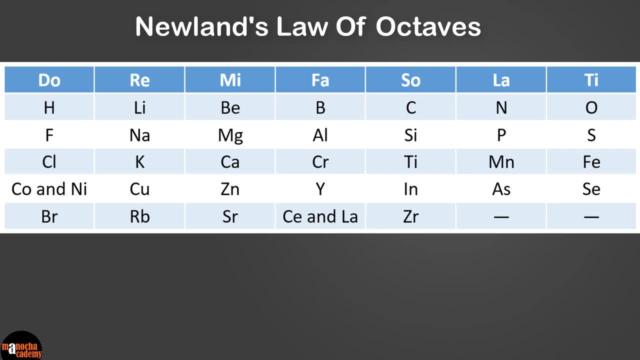 Newlands arranged the then known elements in a table which looks something like this: The elements are arranged in order of increasing atomic mass. The lightest element, hydrogen H, is the first And the last one. The 56th element is thorium. 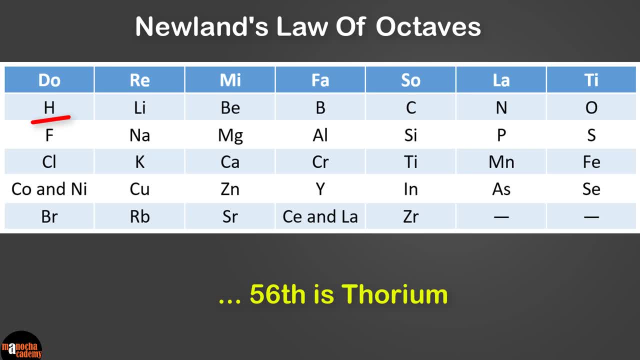 Thorium is not shown here, since this is only part of the table. As you can see, each row has seven elements. Newlands found that every eighth element had properties similar to that of the first element. For example, let's consider the second element, Li lithium. 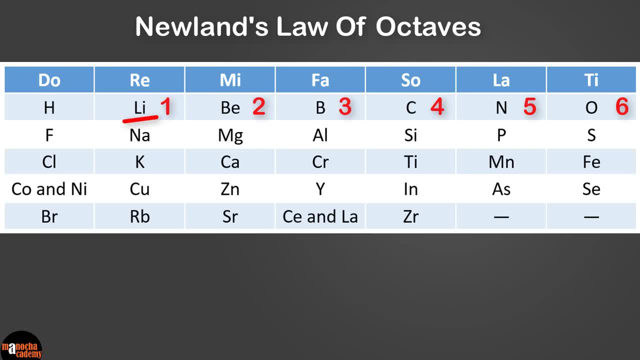 Now, if you start counting from lithium, then the eighth element is sodium, And that means for both, sodium is two and potassium is only one. This gives you a relatively good answer. We fly to a function of the last one and count back. 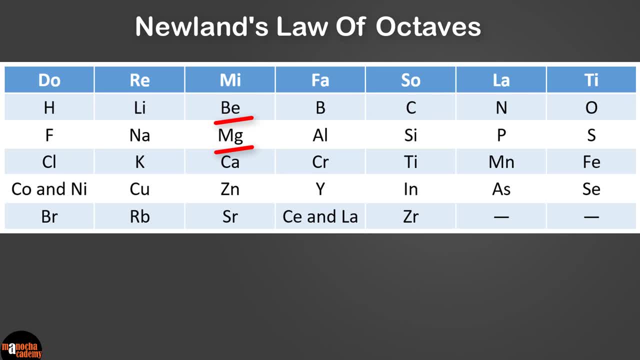 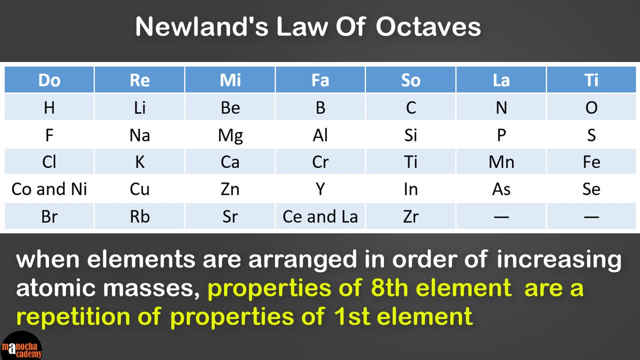 Next, let's Спасибо. Let's Maybe Ottawa, Thank you. Thank you a lot. Thanks for your question, Well done. calcium are also similar. So according to Newland's law of octaves, when elements are arranged in the order of increasing atomic masses, the properties of the 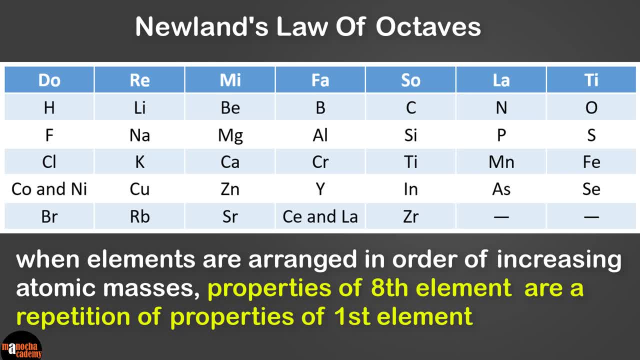 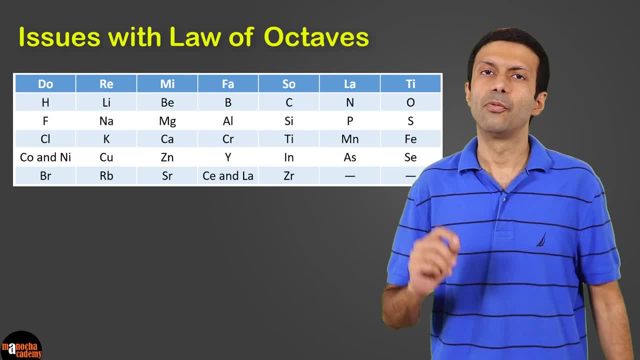 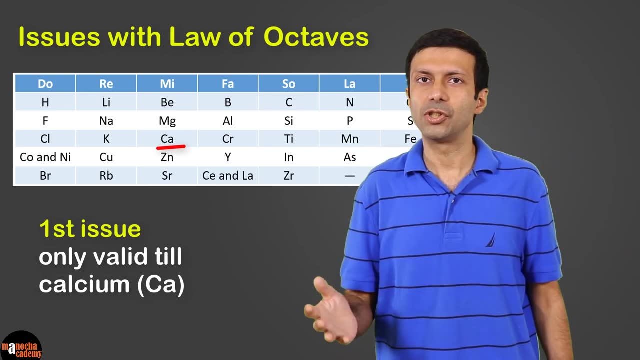 eighth element are a repetition of the properties of the first element. Now let's take a look at the issues with Newland's law of octaves. The first issue was that the law of octaves was only valid till calcium. So after calcium, the 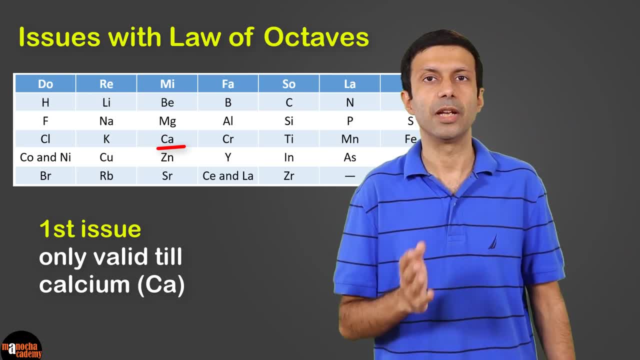 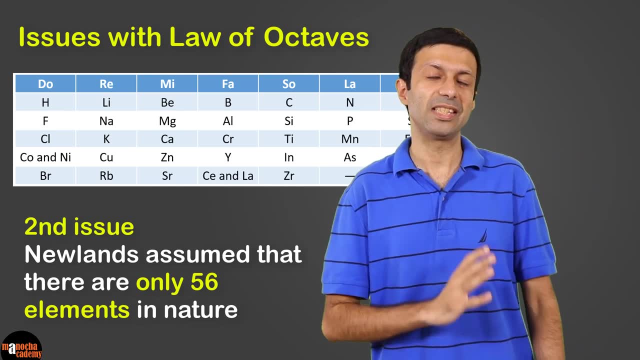 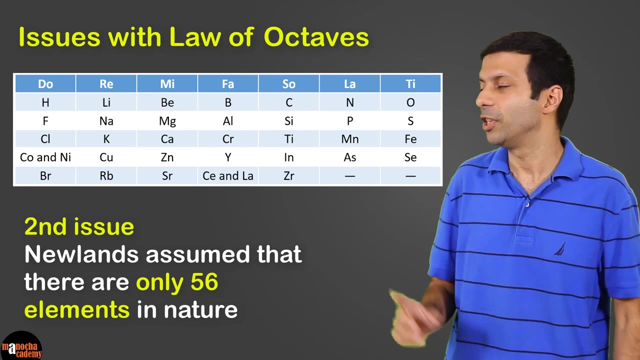 eighth element did not have similar properties compared to the first one. The second issue was that Newlands assumed that there are only 56 elements in nature And later, when more elements were discovered, their properties did not fit into the law of octaves. And for the third issue, let's take a closer look at. 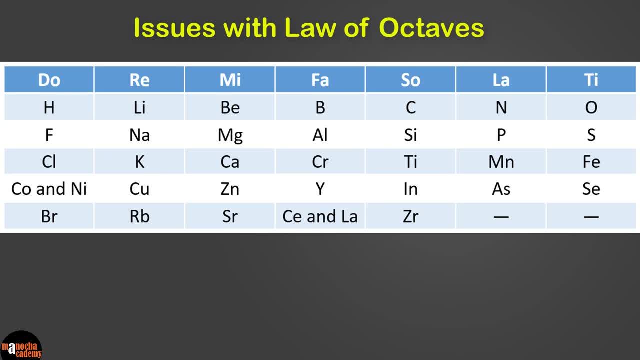 his table. The third issue is that, in order to fit elements into his table, Newlands put even two elements in one slot. As you can see in the table here we have cobalt and nickel, CO and NI in the same spot, And cerium and lanthanum, CE and LA. 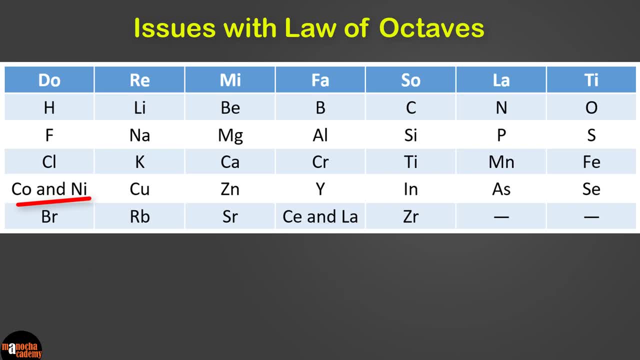 here, also in the same column. If you look at cobalt and nickel, they have been put in a column of elements such as fluorine, chlorine and bromine, which have very different properties compared to cobalt and nickel Iron, which resists.